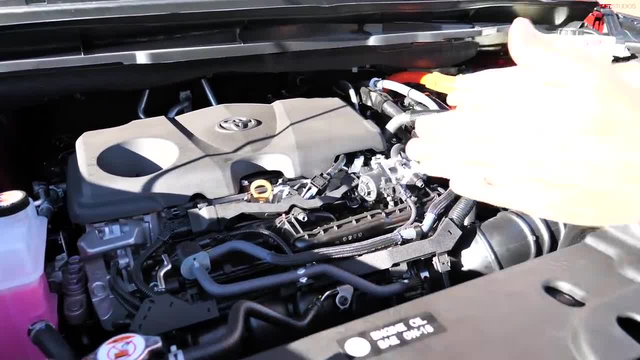 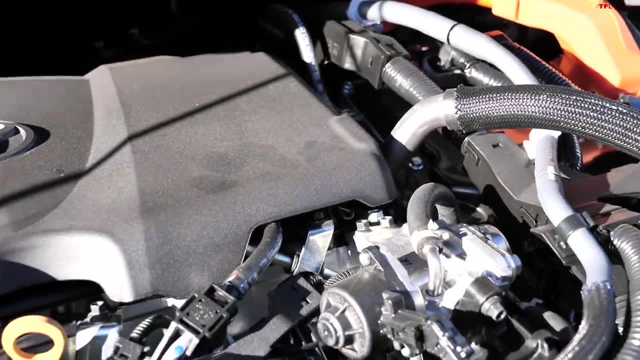 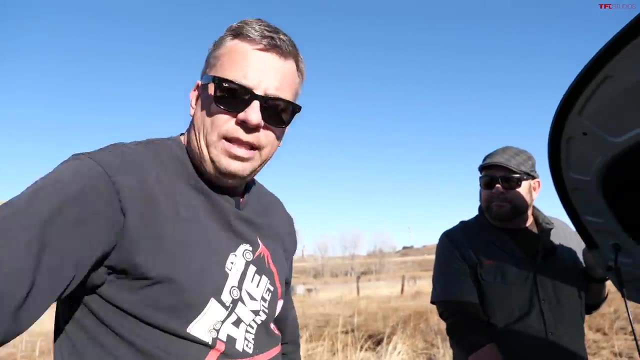 but they're way super different in power, Because right here it's all hybrid technology. all the time It's a gasoline motor, four-cylinder in this case, made it to electric motors And combined 245 horsepower, Nathan, And also capability of all-wheel drive in the Sienna. 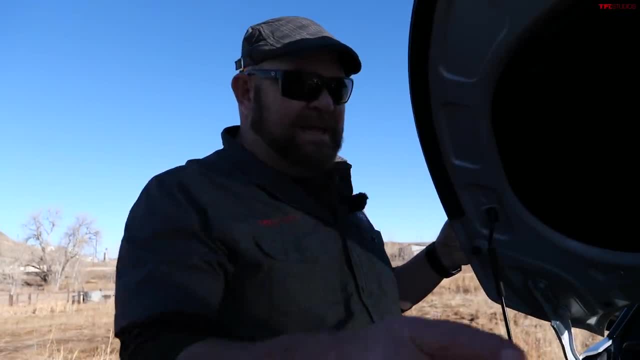 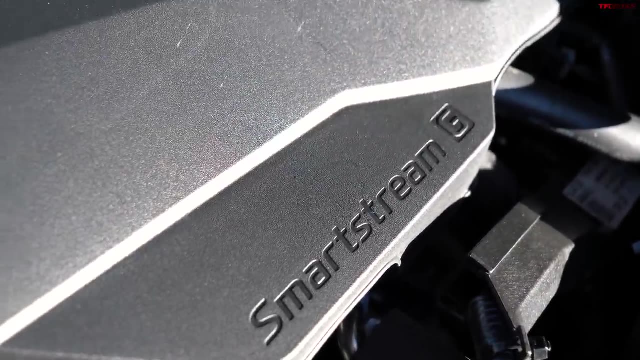 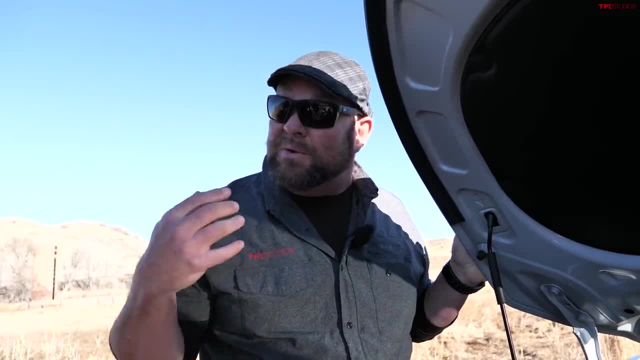 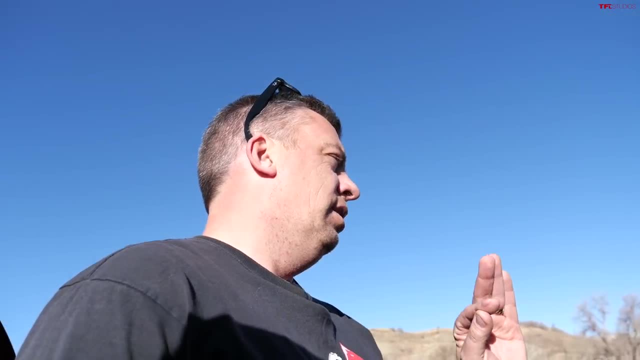 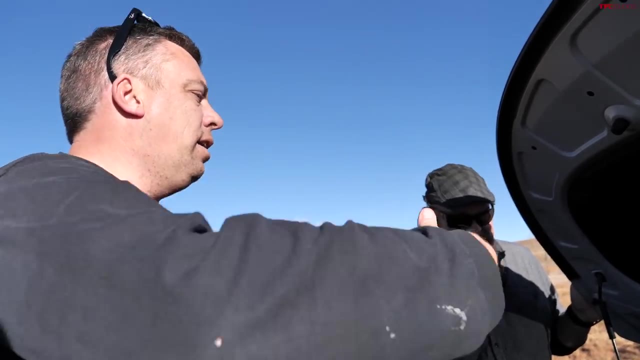 Ah, I have an eCVT, Right right, I'm only fading the front wheels. There is no option in this vehicle for all-wheel drive, So your whole thing about this looking like a crossover or an SUV kind of falls apart because you don't have four-wheel drive. Yeah, and I have a theory about that. I think that Kia specifically did that because they don't want it to compete with their crossovers, But the best number here is 35 combined MPG, which is mind-boggling considering how big and heavy this machine is. 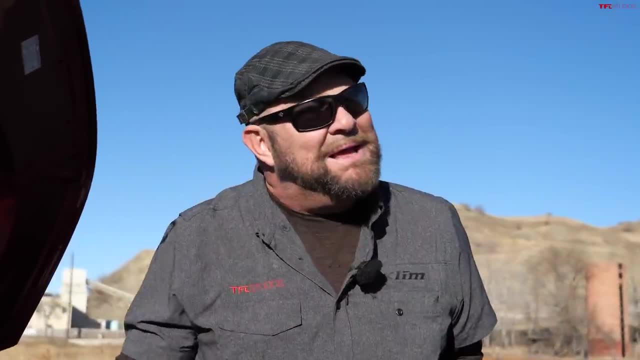 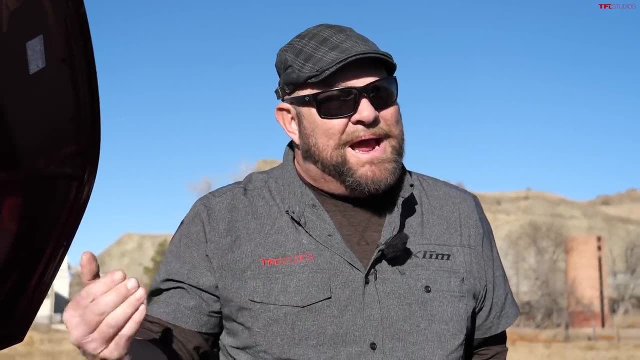 Yeah, I maintain that all minivans should be plug-in hybrids or, like this, a regular hybrid, Because, think about it, families want to move around, you want to save money right And also move in the city Precisely. Unfortunately, mine is not as efficient. 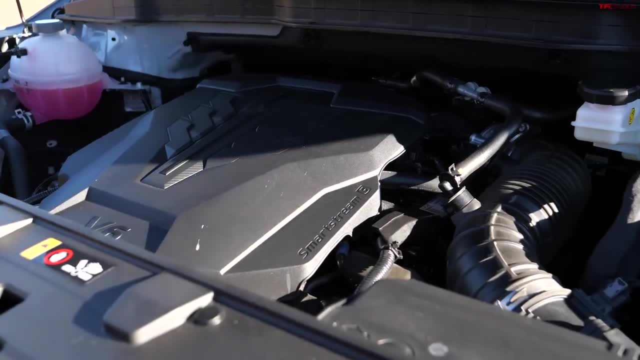 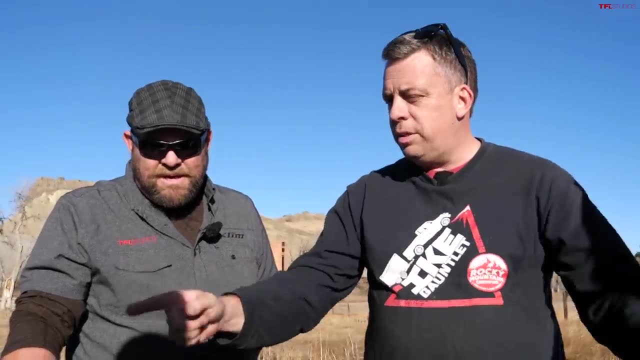 Mine is a regular gasoline engine putting out 22 MPG combined, But we have to do something. We have to do something else. How about we take them on a short drive, Because I bet you, the driving experiences could differ, Completely different. yes, 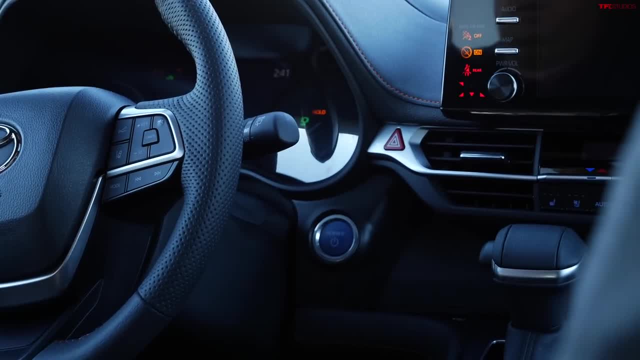 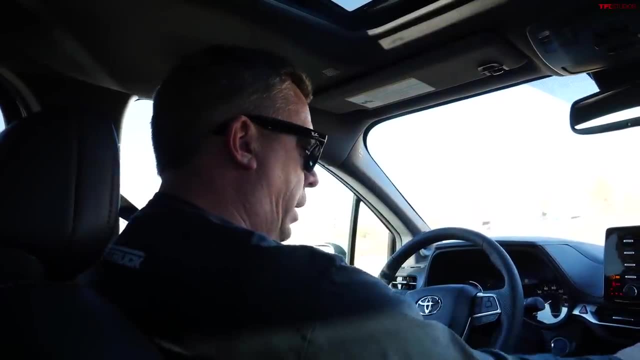 I'm going to power up this machine. No, no, it gave me one beep and now I'm in electric mode, which means I can gently pull away. Let's say it's early in the morning, My family is asleep. I don't want to disturb anybody. 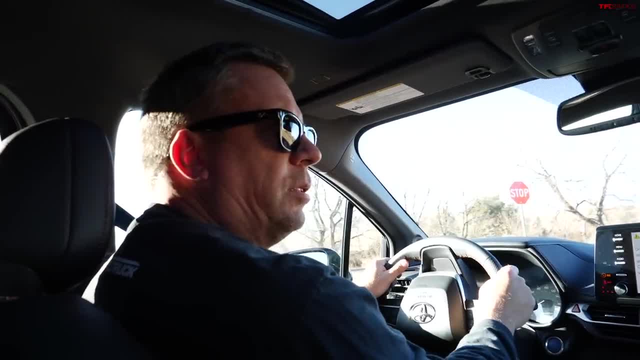 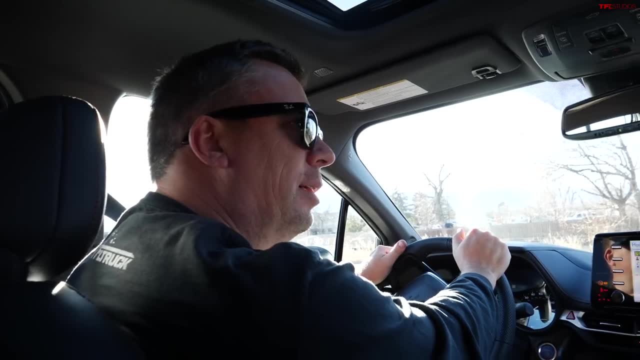 And I just gently waft off to work. I want them waking up with a fright Just hearing me going That way. they know oh, dad's leaving to go win bread for the family. Okay Well, all right, Let's see how it accelerates. 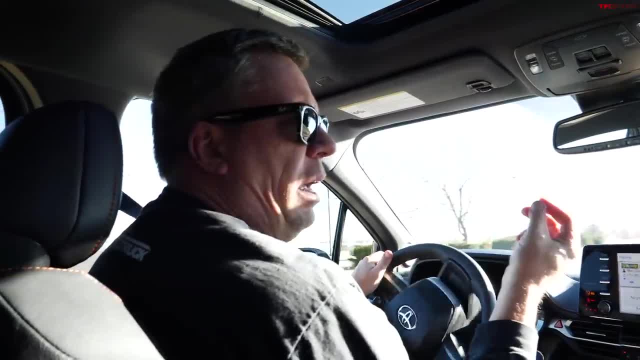 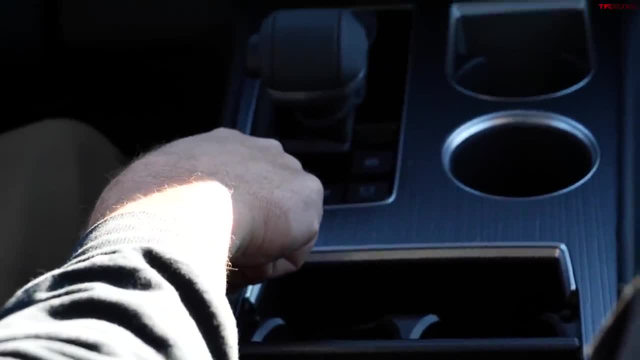 Okay, Because, yes, that MPG number is amazing, Right, But it's almost unbelievable. Drive modes are right here by the gear lever. Okay, little switch, I have sport. Yeah, I have eco. How about sport? This is a sporty review. 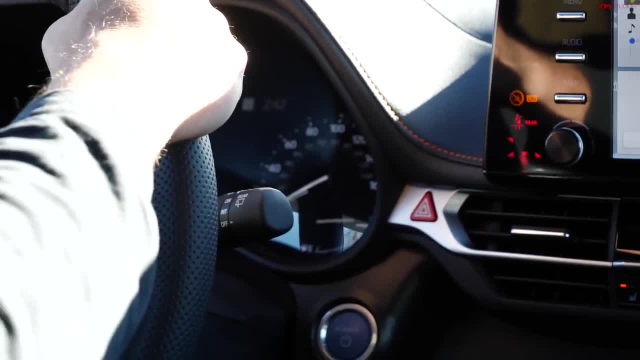 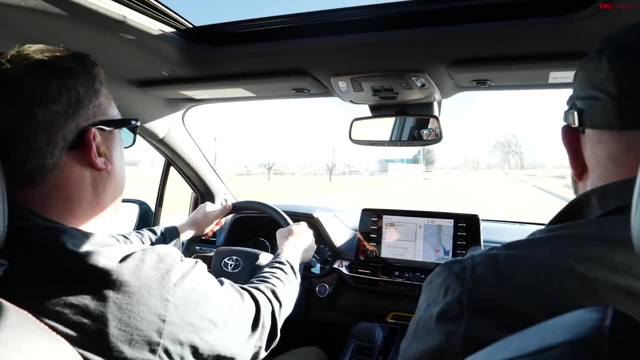 Yeah, sporty time. Are you ready? Yep, Hit it. Whoa, The power is overwhelming. No, it's not really overwhelming. No, it's not, It's a minivan, but actually it gets up and goes. 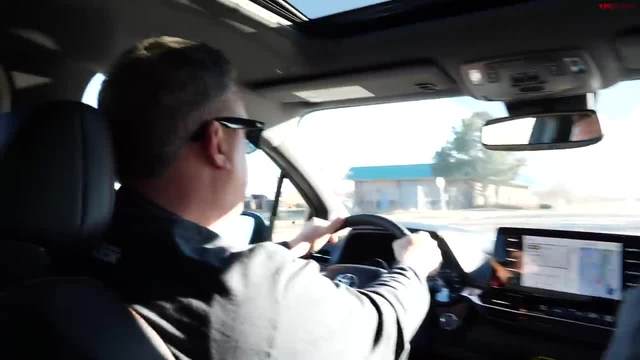 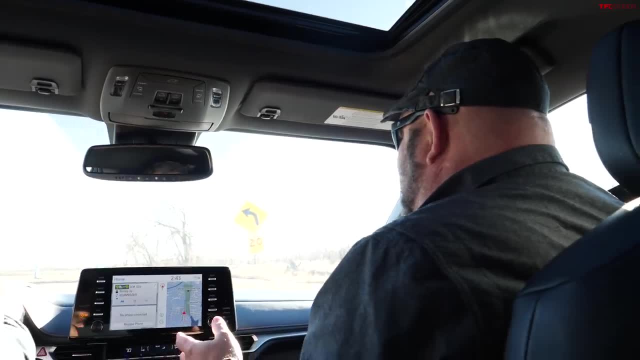 Yeah, So that's 60.. Yep, So that took, well, I don't know, six or seven or eight seconds, Regardless of what it takes, And we've actually put this thing on the solo DL before, but it does have all-wheel drive and the all-wheel drive system makes it fantastic in snow. 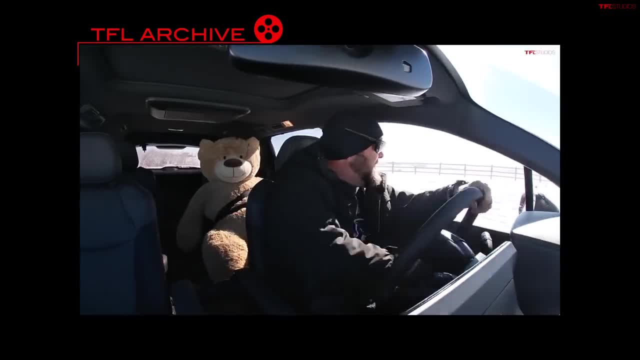 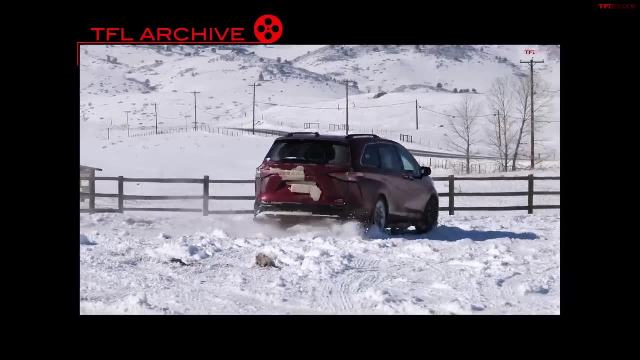 We actually have a video showing that, So people can either go to alltflcom or, more specifically, search on YouTube. Yeah, They're going to have to search on YouTube. TFL, Toyota Sienna all-wheel drive- Right, Because it's too late. 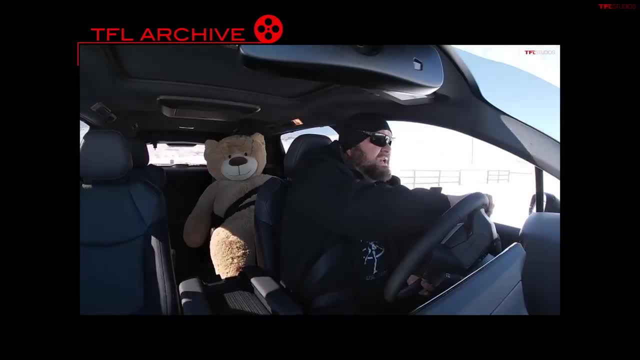 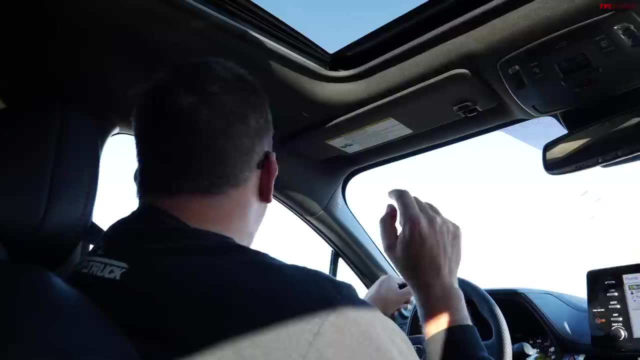 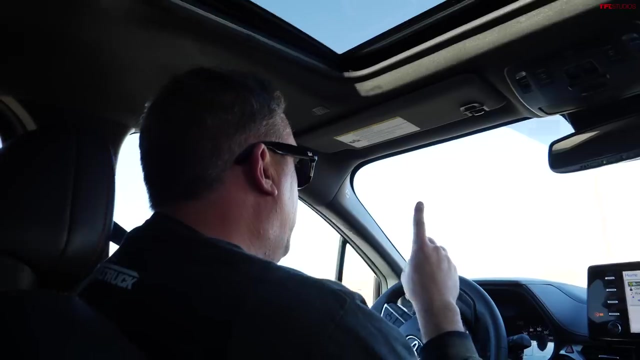 That review was over a year old. Yes, It won't show up at the top of our feed, But here's the thing. The transmission, the ECVT, electronically controlled, continuously variable transmission, That's Toyota talk. Yes, It's very efficient, but it's droney. 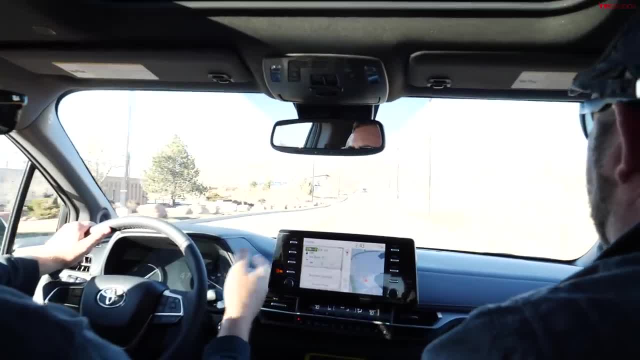 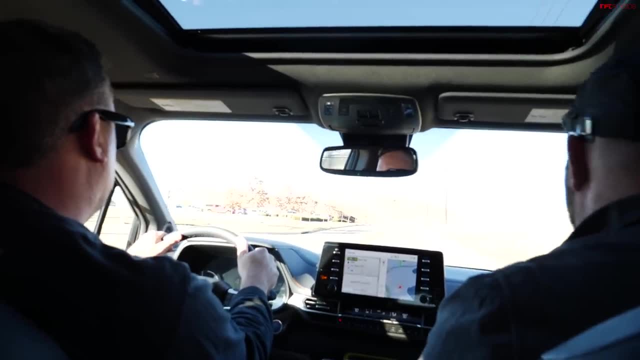 Yeah, It's just going to sit at that RPM until it knows that you no longer need that much power in the drop. Yeah, It's a very different feel than your average car. However, if you drive it normally, not with a lead foot, it's not that bad. 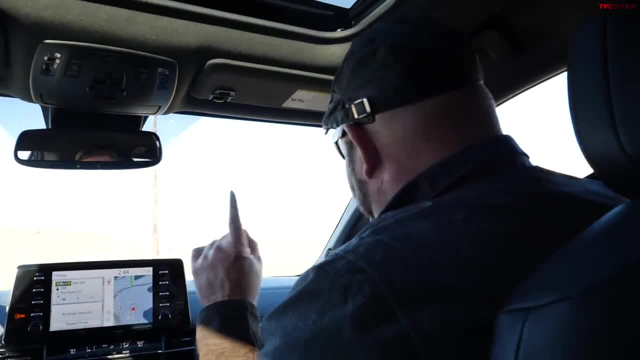 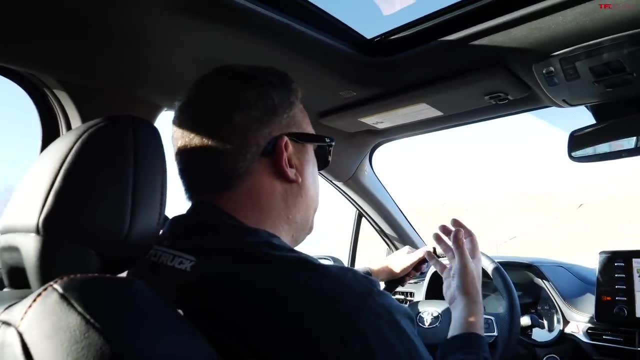 But, Yes, Can you hear the outside noise? Yeah, A lot of the outside road noise and these expansion joints. I can feel that through the canopy, Yeah, They're coming through a little bit here And this is not a basic Sienna. 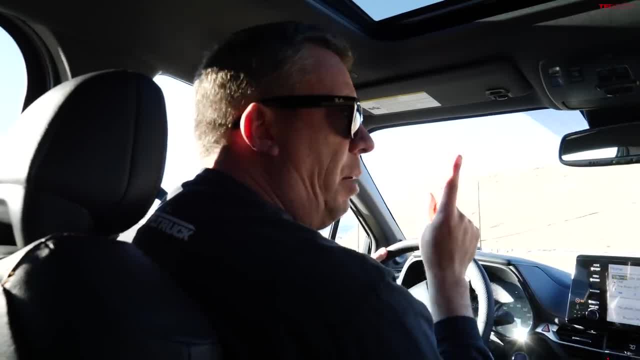 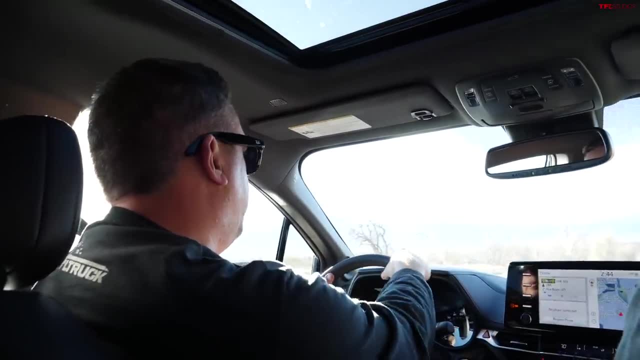 This is an XSE all-wheel drive with a couple of options. That is correct. So it's on the nicer end, but it's definitely not the very top. I feel a little bit Removed from the driving experience because the steering I don't get a lot of feeling. 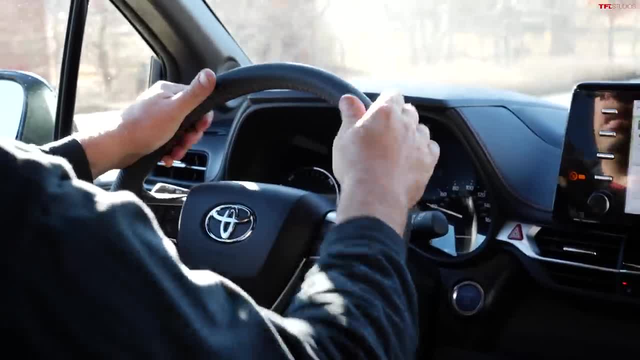 from it at all. It's pretty light, isn't it? Yes, It's light. There's not a lot of feeling, but it's a people mover. This is kind of, I think, par for the course, isn't it? 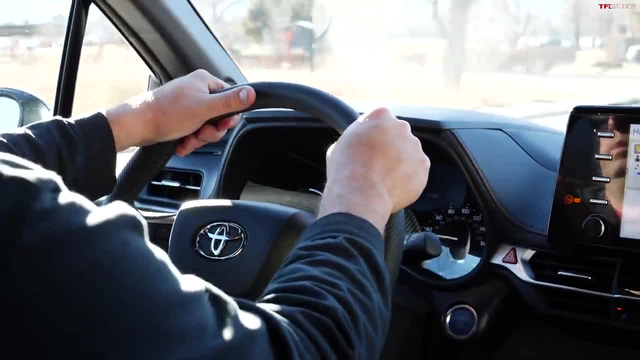 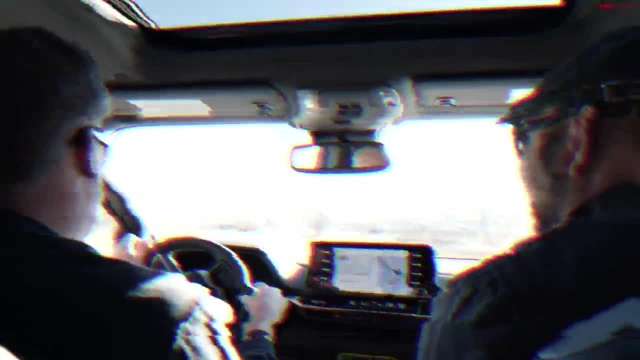 I would agree a hundred percent. And, in addition, that all-wheel drive system is completely seamless. It does everything it needs to do on its own, and it will help you enhance your driving in general as well. All right, Let's fire up this Kia Carnival. 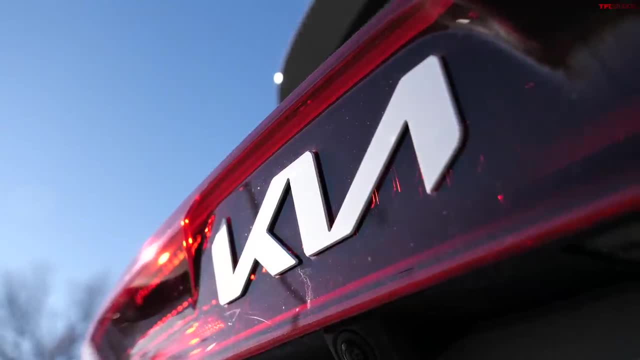 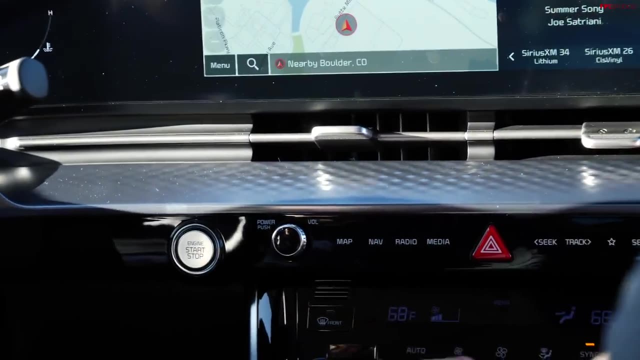 Is that how you say it, Carnival? I feel like I'm in a More premium vehicle for some reason. I mean just feels a little bit nicer. Look at some of the stuff that they're putting here like this, you know, going across. 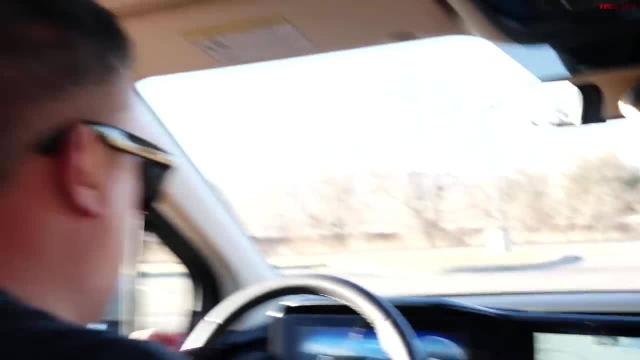 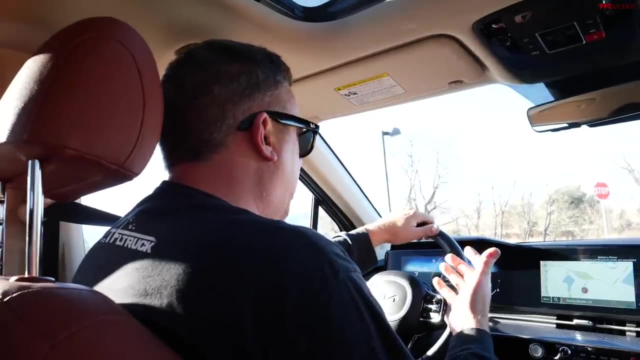 We'll go over that a little bit later with our very special new feature that we're going to be talking about. But, yes, the seats are already much more comfortable. But it's a traditional vehicle. So if you're used to regular automatic transmissions and regular V6s, this is your jam right. 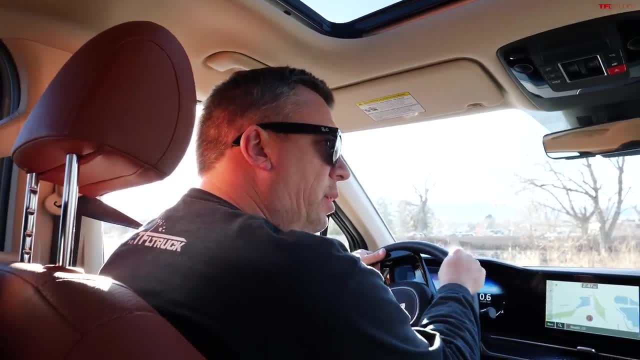 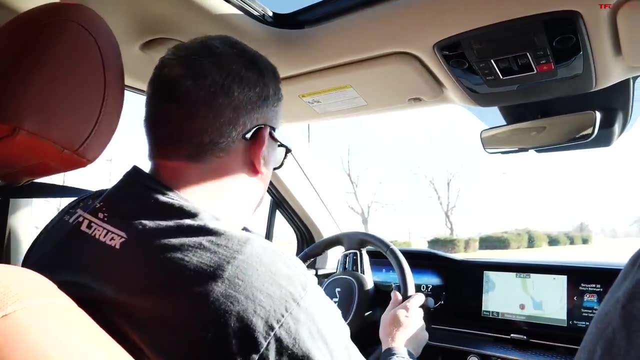 That's what I'm talking about. Okay, And this is more power. So you said it had more power, So I want to put it to the test Now. unlike, well, you go ahead and accelerate. Oh yeah, Here's the tape measure. 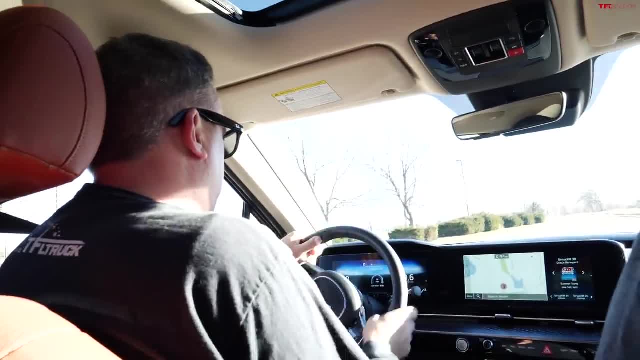 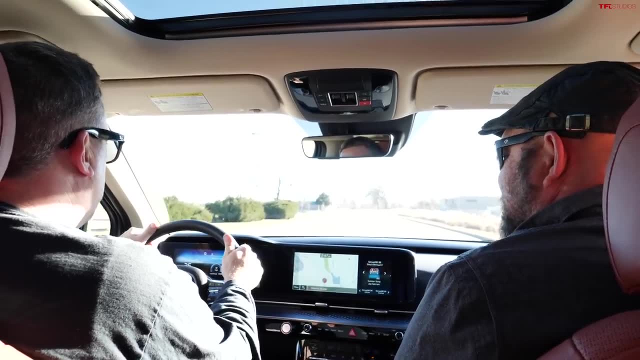 Here's the tape: Perfect, That's for later. That is for later. Ah well, you know this is also not a speed demon. No, it's not, But it is. It feels quicker, at least Bam. 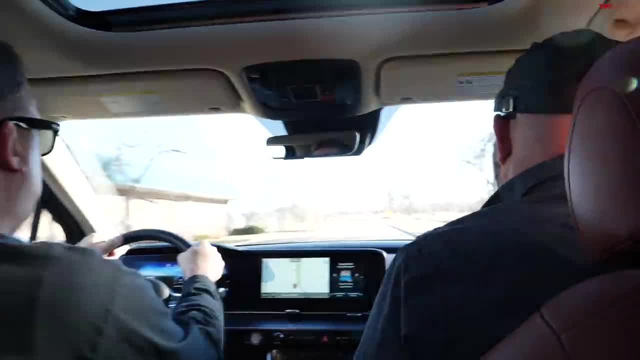 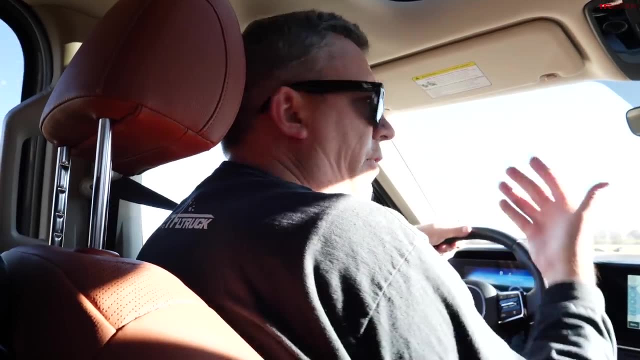 Yeah, That was 60. So it feels quicker to me. It is also more auditory, You know, kind of pleasure, because you can hear the gear changes, You hear the V6. Which is very smooth, by the way, Yeah. 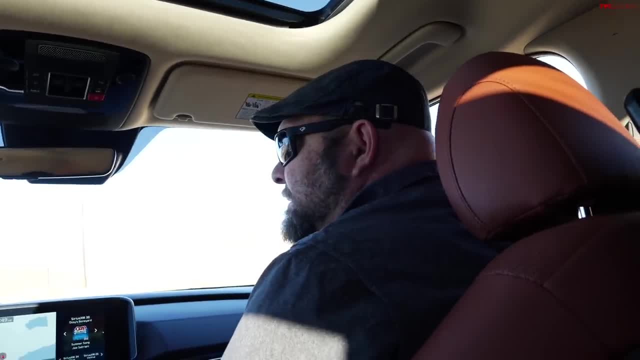 Can you tell- at least the seat of your pants- the difference in terms of ride quality? It feels a little bit more solid And definitely the steering is a little bit heavier. Yes, it is, And I feel a little bit more kind of engaged. 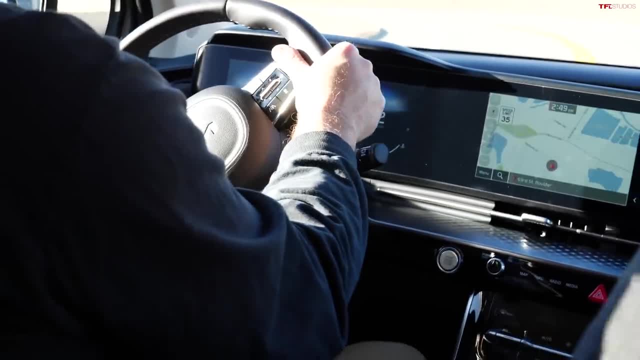 I would agree with that as well. I think that the noise isolation is slightly better in this, Although- feel this in the corner- It leans a lot more, doesn't it? It does lean. I think that's the softer suspension setting. 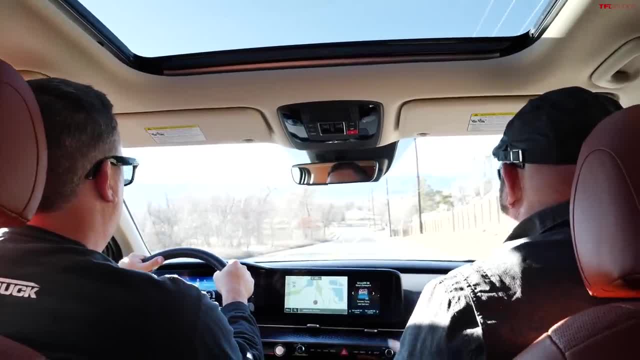 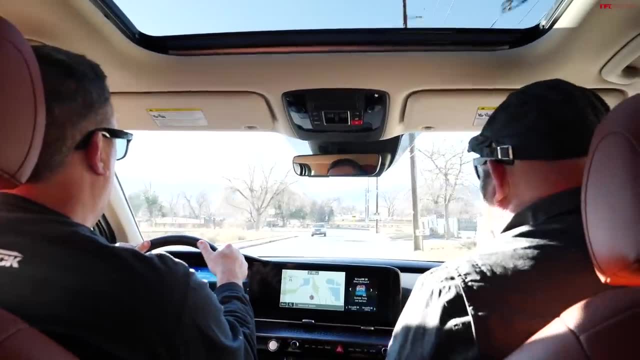 Uh-huh. So that's definitely a difference right there. So once again, it's a bit of a mix, you know, between the two of them. One of them is a little tighter and a little noisier, But it seems, at least around the corners, not to lean as much. 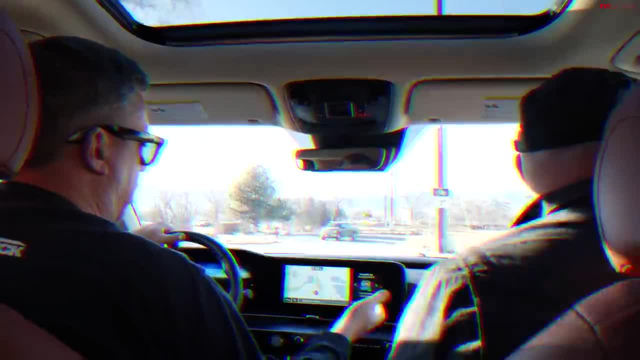 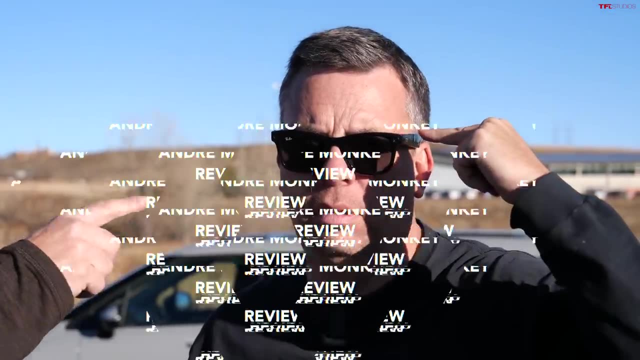 This one is much smoother But at the same time leans a lot more in the corner. Ladies and gentlemen, I want to introduce you to the Andre Monkey. The Andre Monkey is very special because he's wearing special sunglasses that have cameras in them. 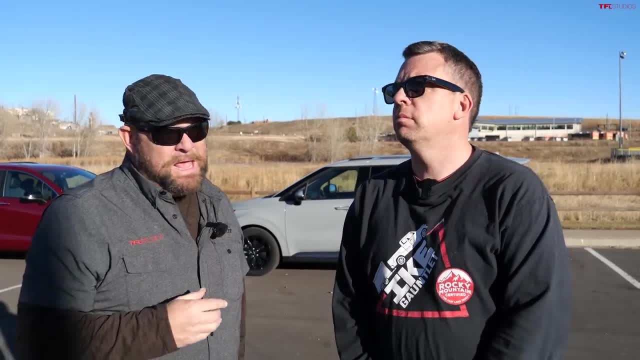 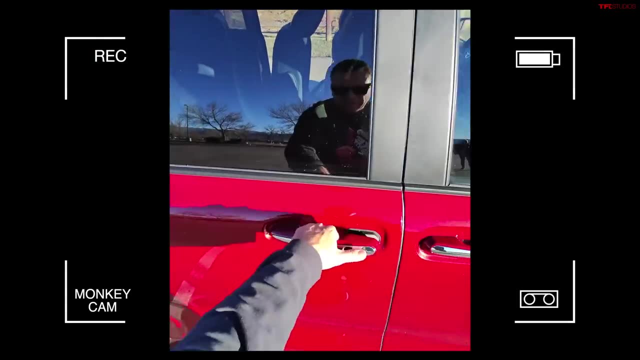 And he is going to explore the interior of this vehicle, And if this is successful, the Andre Monkey may return in another video. It's up to you. All right, I want to check out the center row and then the third row behind it. 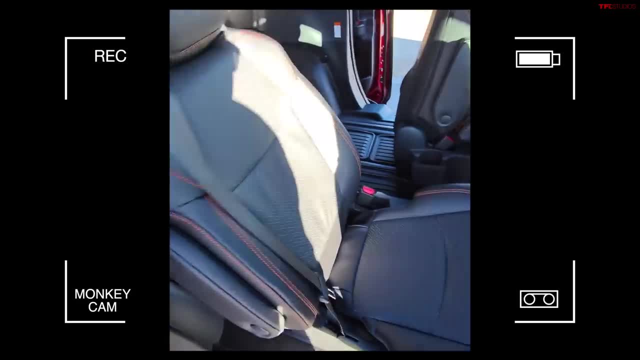 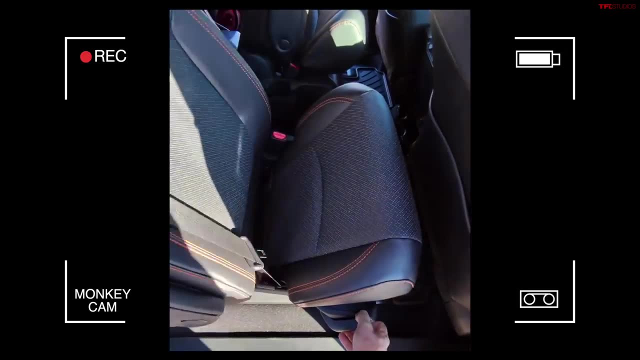 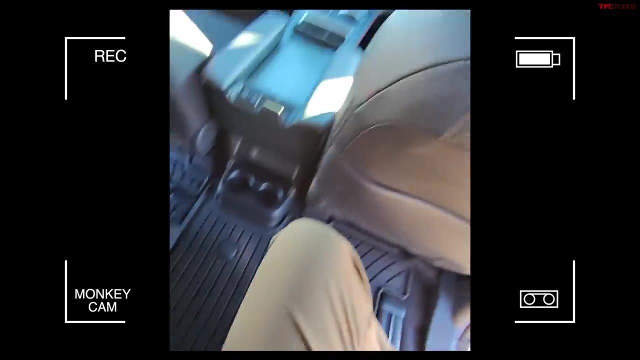 Of course, both power doors And this can recline. This can actually put away this way so I can enter the third row, Or I can move it this way to sit in and enjoy myself. So let me see how far does it go. 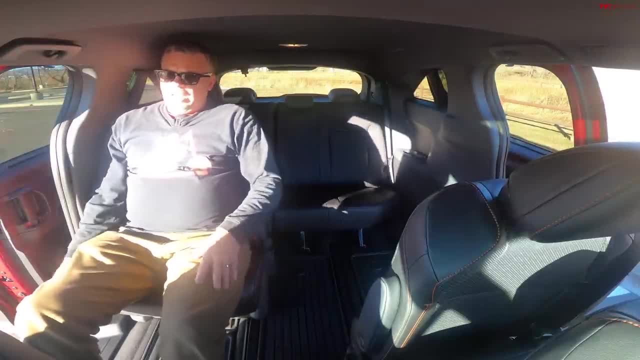 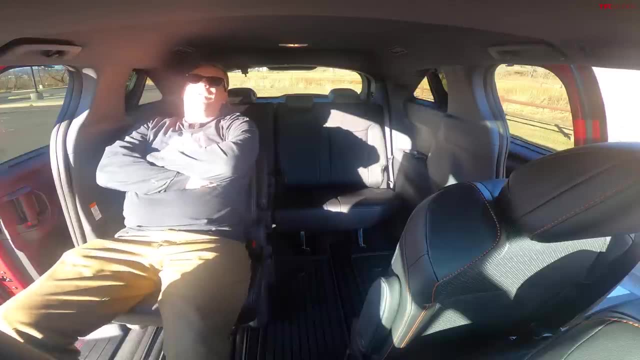 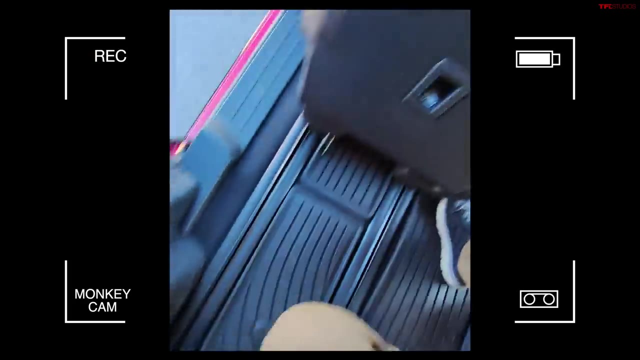 Whoa. So if nobody's in the third row, I can slide all the way And I can also recline. Actually, yeah, this is why you buy a minivan instead of an SUV. This is pretty sweet. Then, since there's this configuration of seven person, I can sit in the third row. 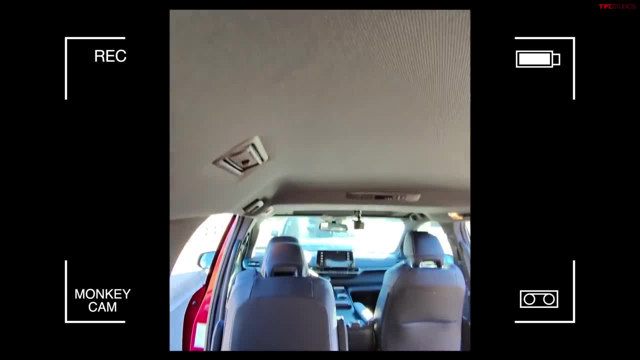 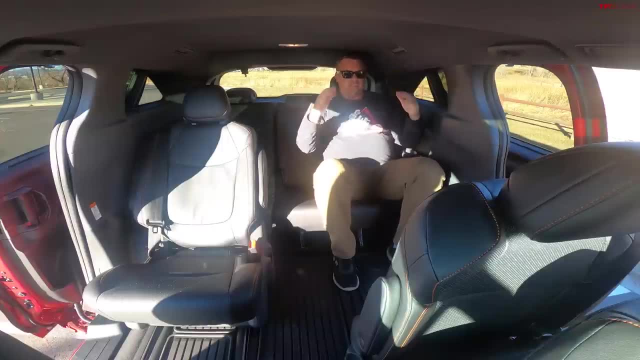 I can move this up, Okay. Very limited headroom And my knees are sticking kind of up, So I think this is for smaller people. I'm just about 6'3". All right, Let me try the Kia Carnival. Once again, both power doors. 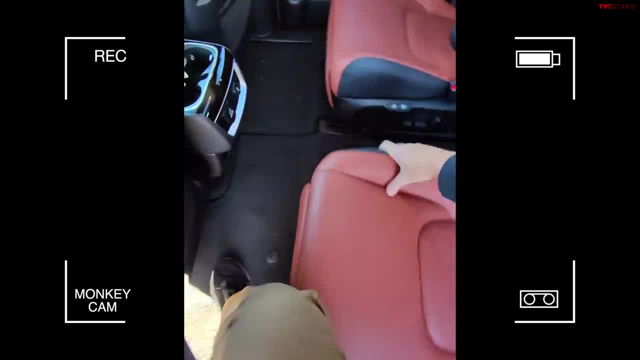 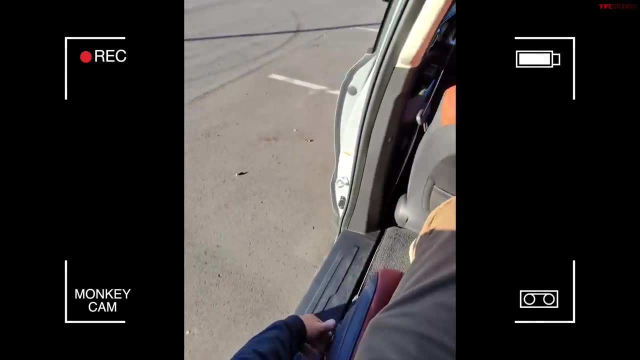 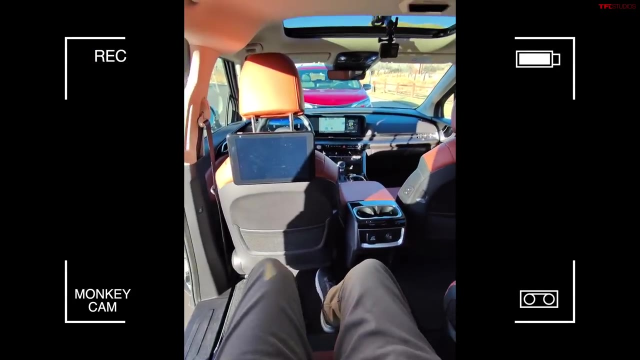 But this has something that's called rear power, VIP captain chairs, which I'm very curious about. So of course it slides back and forth, but has an additional feature: Slides sideways. Oh yeah, And then that allows me to slide all the way back, just like the Sienna does. 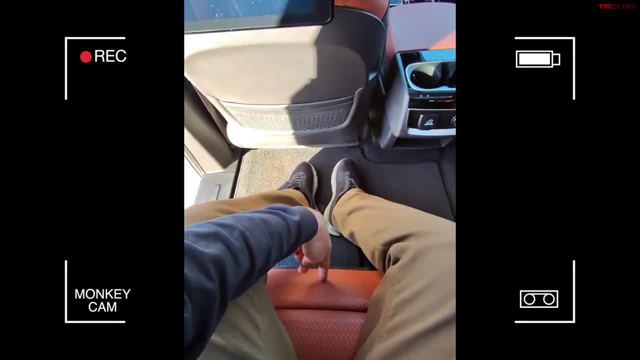 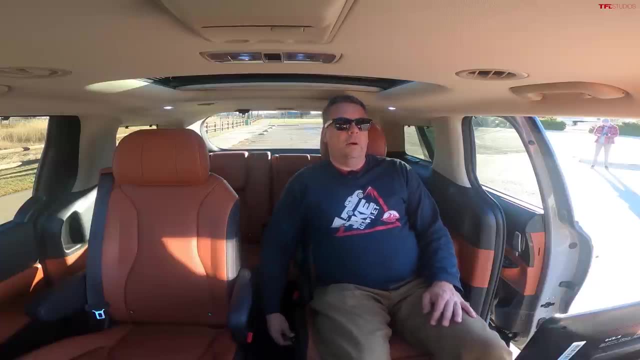 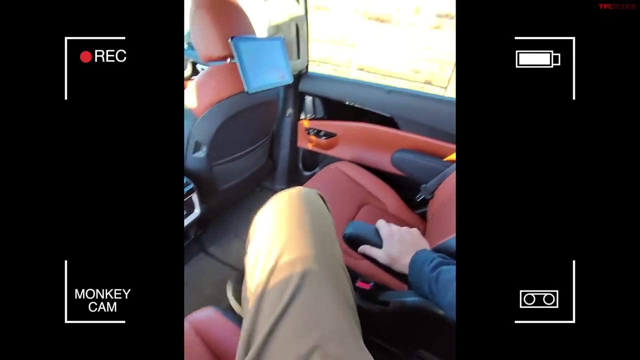 But now I have power features here. I have a power extending footrest And recline features here. Wow, Okay, Now if I wanted to put it back away, I slide forward, slide back. Then I enter the rear seats, which is a little bit harder to do. 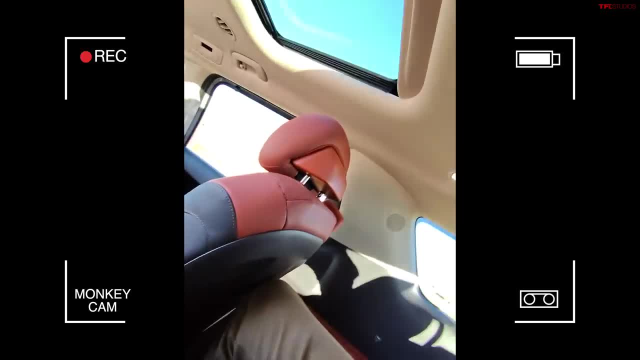 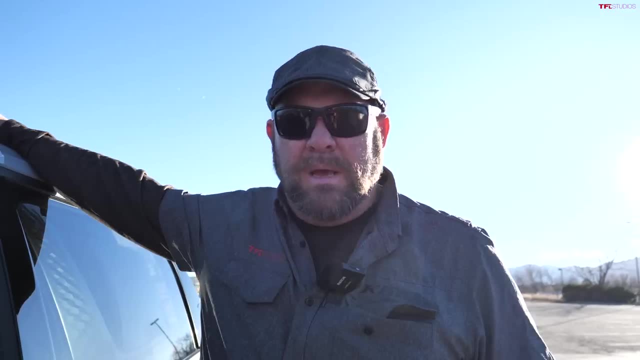 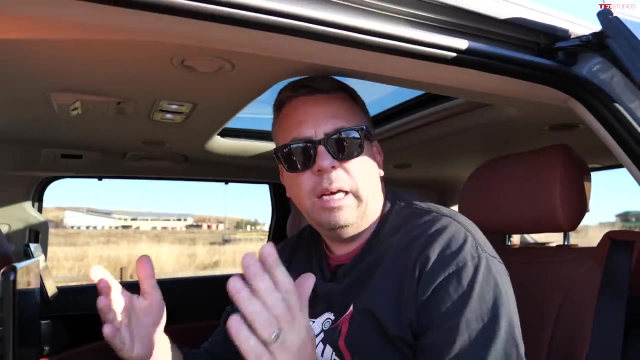 And I actually have cupholders, but I have very limited headroom and very limited legroom. Okay, How was it Eye-opening? Eye-opening In the Toyota, I felt like, because the seats fold, I could get in the third row very, very easily. 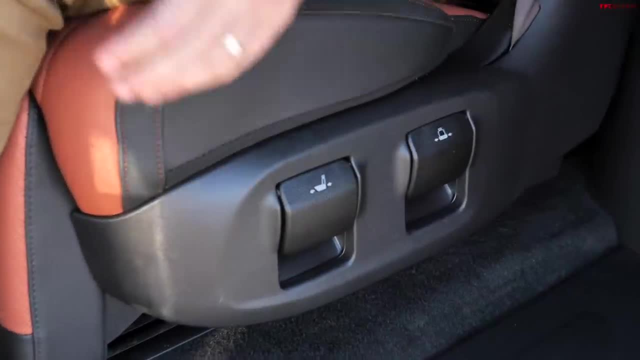 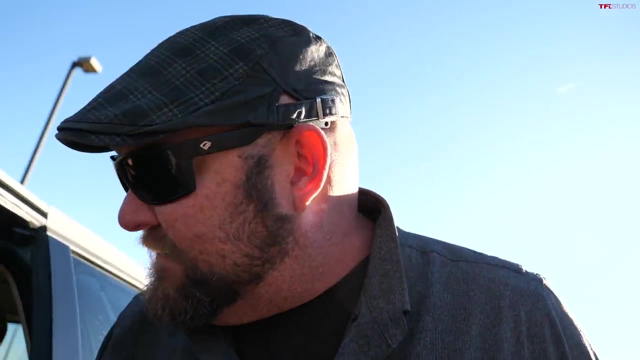 But here, these captain chairs, these VIP seats, make me feel as if I'm in a private jet. Now, bear in mind that Toyota does have an option on their higher-end vehicles to get this cushion to come out as well. Oh, So you get a little bit more comfort with comfortable seats. 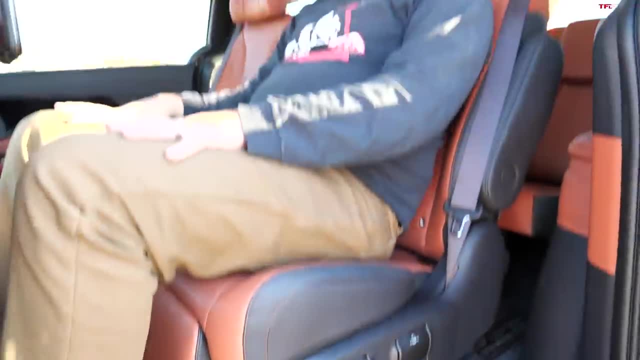 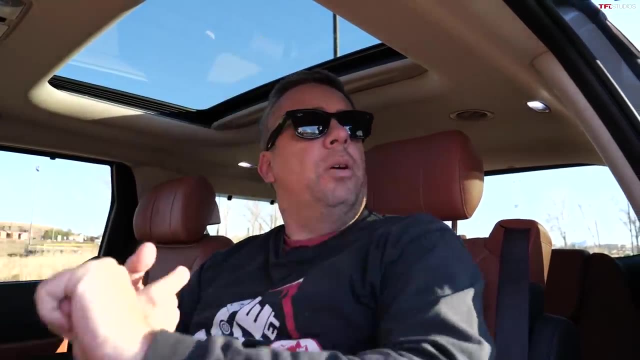 However, these seats do a lot more than the Toyotas do, And you have all that electric stuff going on. Okay, Well, let's talk about more utility, because there is also door size, rear storage of seats and also towing And cargo space. 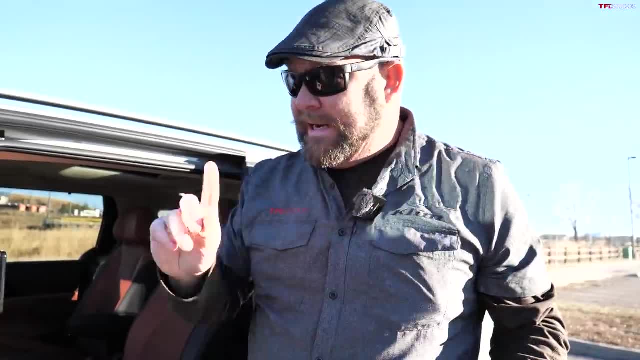 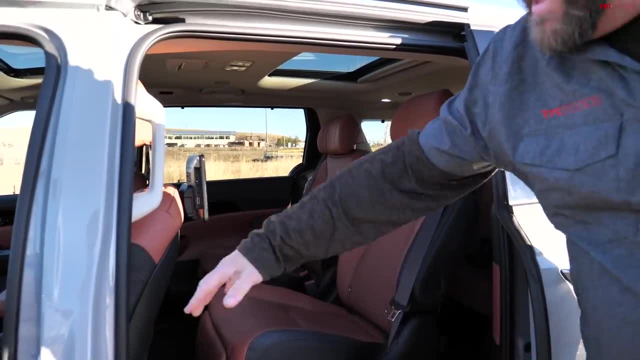 Ooh, All right, Let me whip this out Now. here's an important point: These door openings. some minivans or MPVs have a very narrow section, which makes them less utilitarian. However, some of them have a larger one. 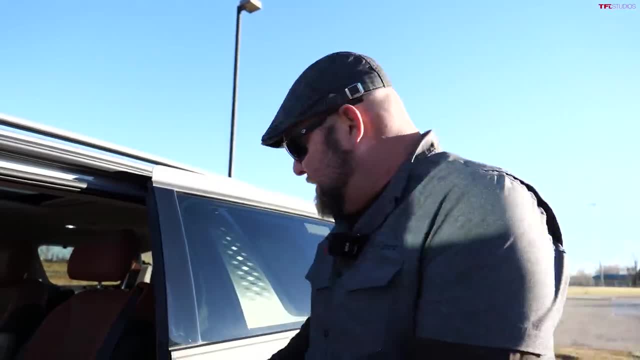 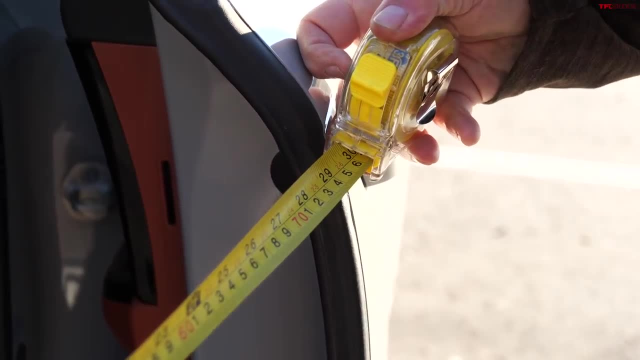 Now I maintain that the Kia's is pretty good, So I'm just going to go and whip from the door All the way open to about mid-level And it looks like it opens at about 29 inches. Let's look at the Toyota from the opening over to here. 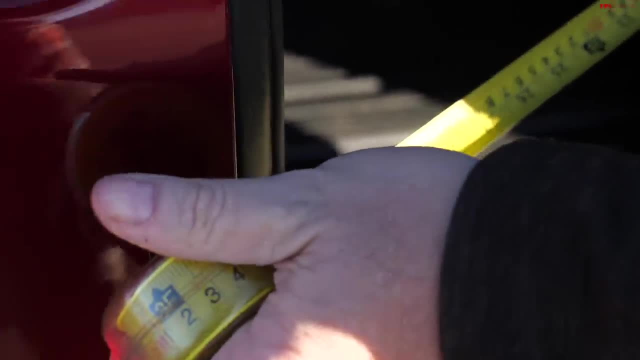 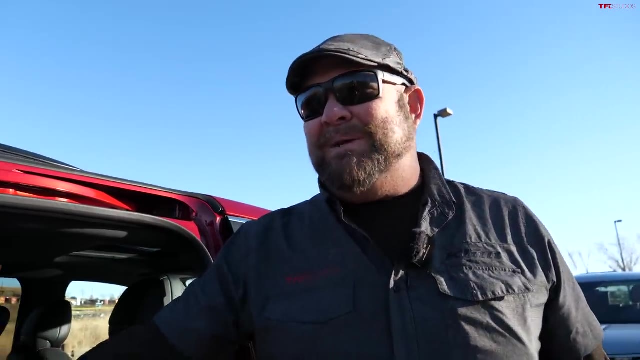 And it looks like the Toyota has got an edge here. that is just about 30 and a half inches, So it is a wider opening. Interesting though, the Kia's doors are a little bit bigger physically, So it's not about the door size. 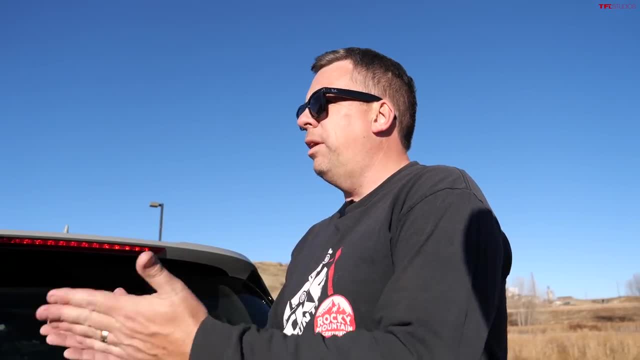 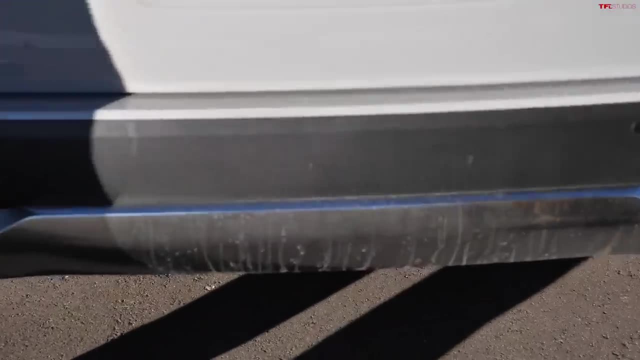 It's about the opening. You know that we do the iGauntlet, World's Toughest Towing Test at TFO Truck. Yes, Can we tow with that? No, because there's no hitch, But there could be. There could be a hitch. 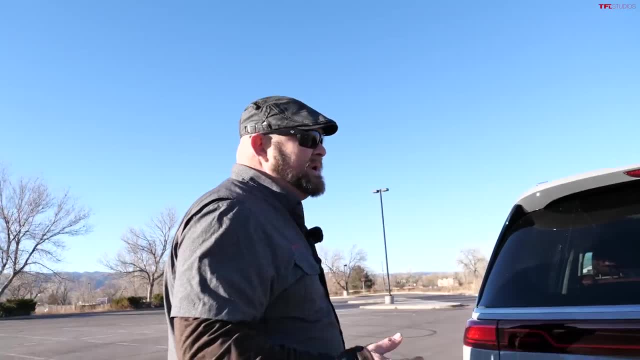 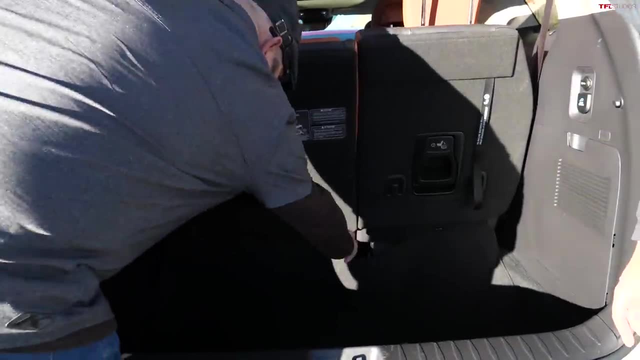 Right, There is a towing package And both of these vehicles are rated at 3,500 pounds maximum. All right, So you could bring a small, tiny like a single axle trailer with you for camping Correctamundo, Okay. 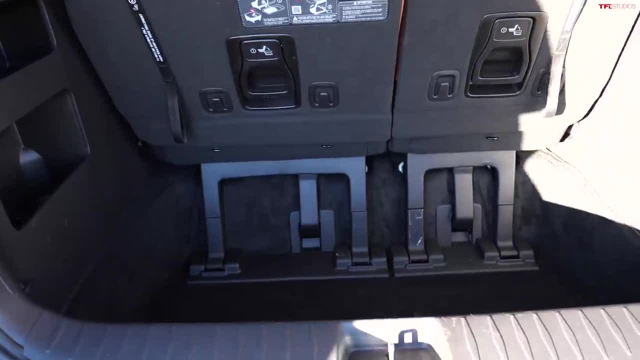 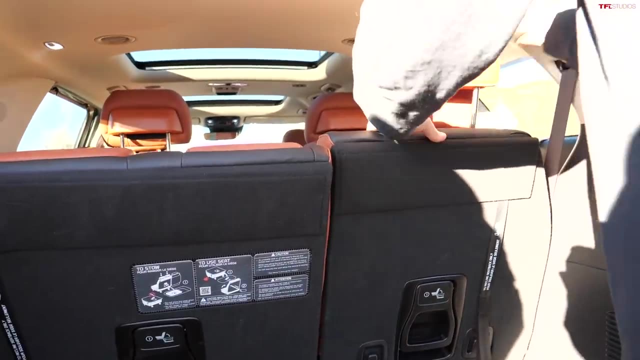 I'm moving this out. This is actually. this is something that you can get later on with Kia, And I'll show you what it does later, But it doesn't work with the seats up, Okay, So let me lower this headrest, because I was moving it up for sitting. 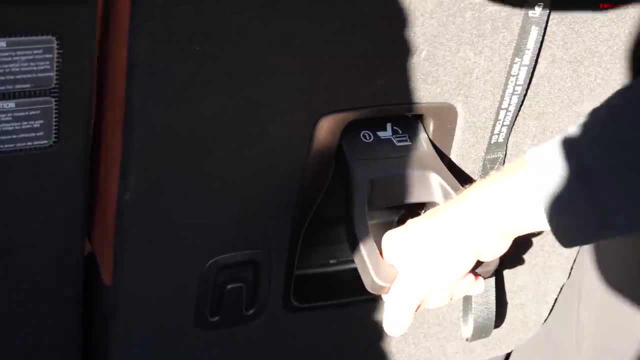 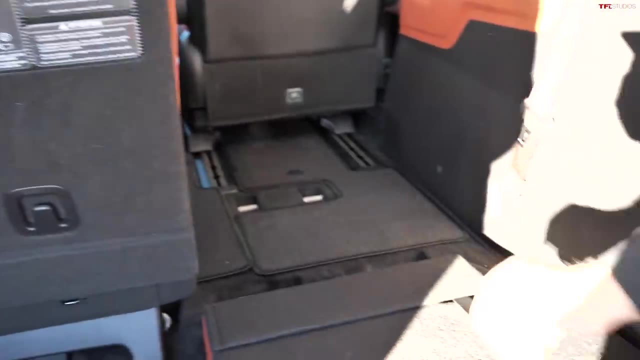 Yeah, Now let me see if I can, Because I haven't done this in a while. The instructions are right here. Oh, even a monkey like me can do it. Right, You got to fold that, though, Or else you don't have a flat surface. 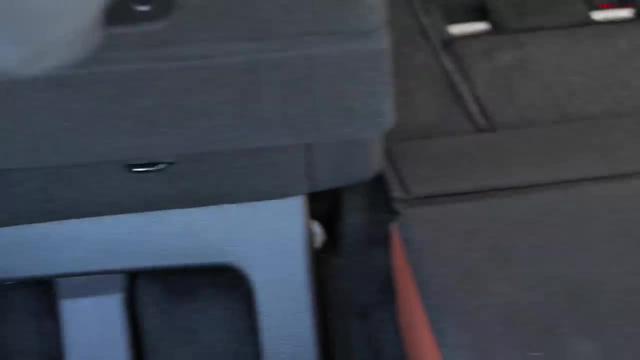 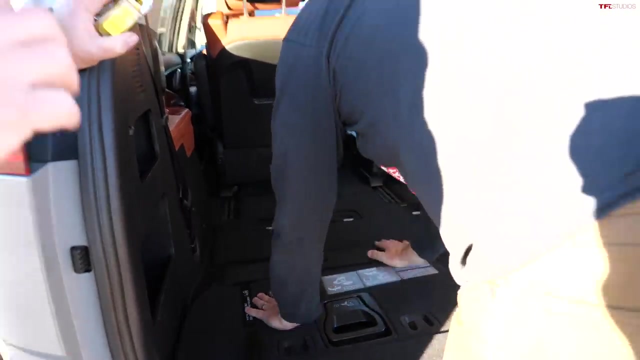 Oh this, Yeah, There you go. Now you have a flat surface. There you go, Good boy, Okay. So this is better than a Bojanca. I would say, Well, anything is Okay. So, while he's holding that down, something that you need to know, guys. 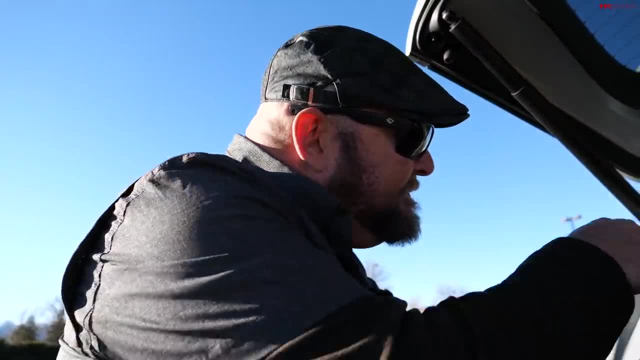 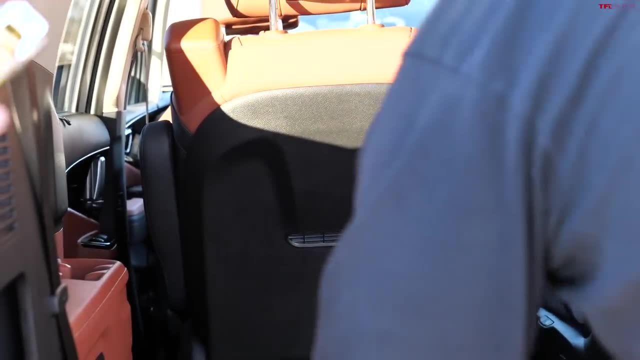 When you pop these seats open, just like the Toyota. Yes, If those seats in the middle are back or reclined, you will not be able to get these up, So you have to make sure that those are slid forward. It's for both vehicles. 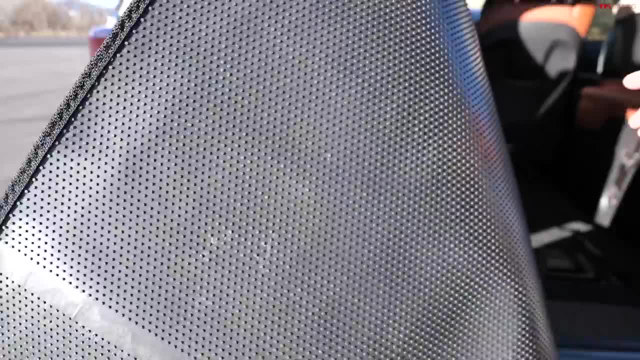 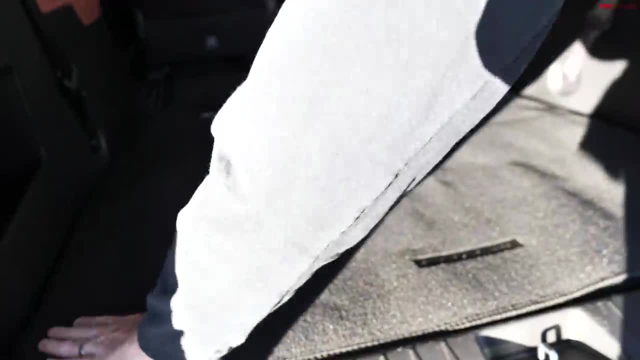 There you go. Now that that's like that. now you can put this in. Okay, So I can cover this up for cargo mode. Okay. What irritates me is that this mat doesn't work anywhere else. So in other words, if we pop these seats out, then I just drop it in the bottom. 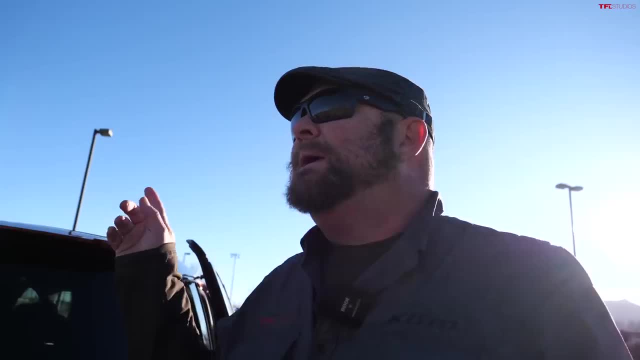 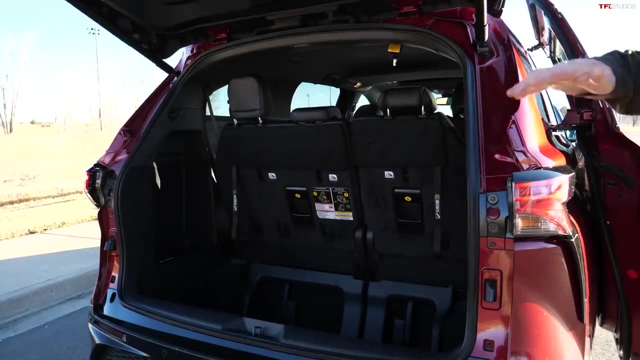 I don't know what else to do with it. It doesn't fit anywhere else. It's kind of a pain. Now we're at the Sienna, You can go ahead and open it. So if you get the woodland edition of this vehicle, it's about a half an inch higher off. 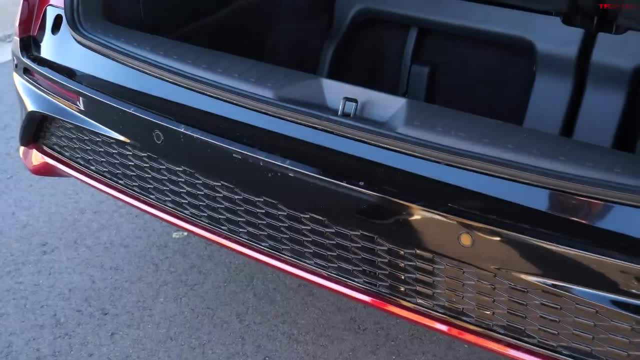 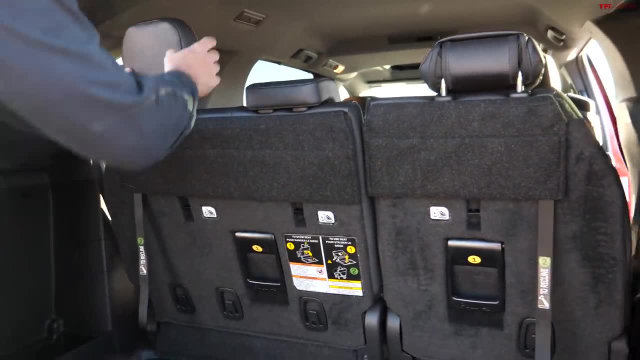 The ground, but it comes standard with the tow hitch Okay Right, But still the same rating. That's kind of nice, Yep. So actually I'm looking at this and this seems like the mechanism is very similar. Yeah, it is very similar. 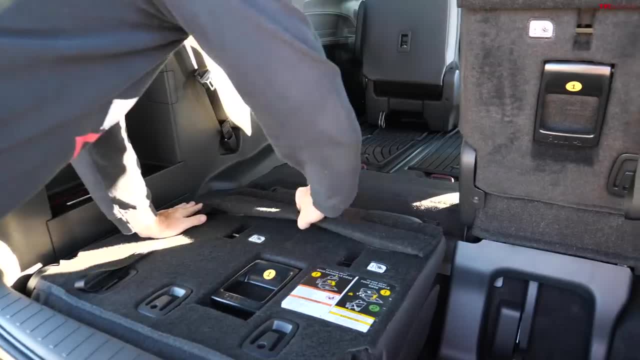 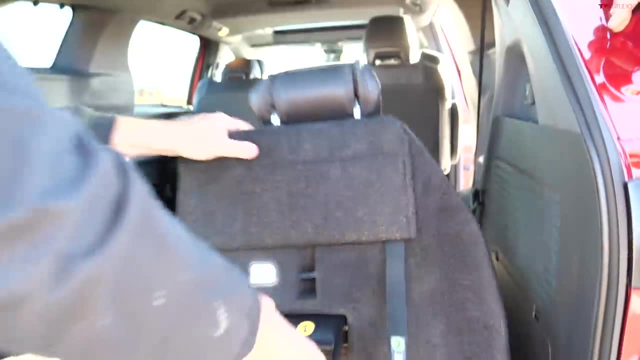 And I think that's a good thing, especially for people who rent these and go to various places and have to get different vans. It's nice to be able to do this. Look how easy that is, I think between you and me, Yes. 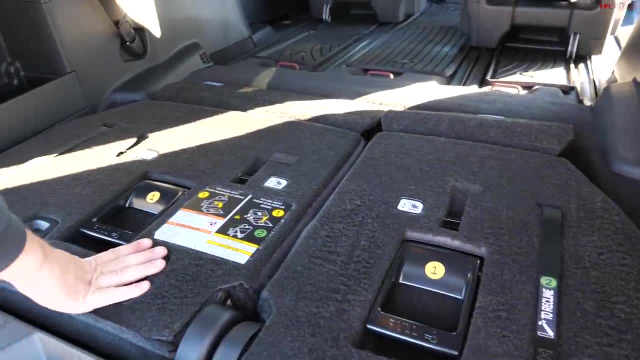 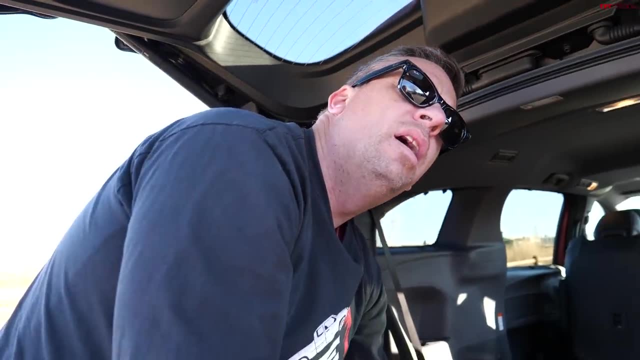 And all of our audience. Yes, This is easier. folding In the Toyota. I had a little bit easier time, but I also have practiced on the Kia, So I'm not telling you, Yeah, But you're going to have to trust me. 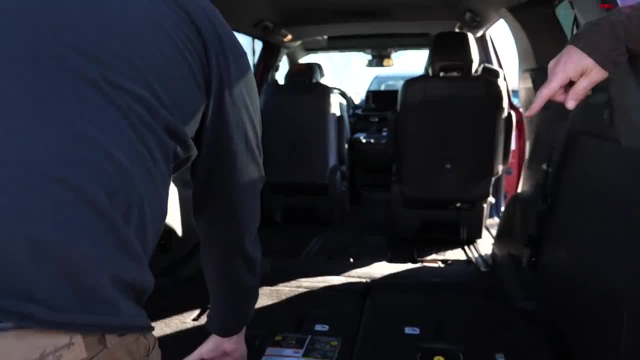 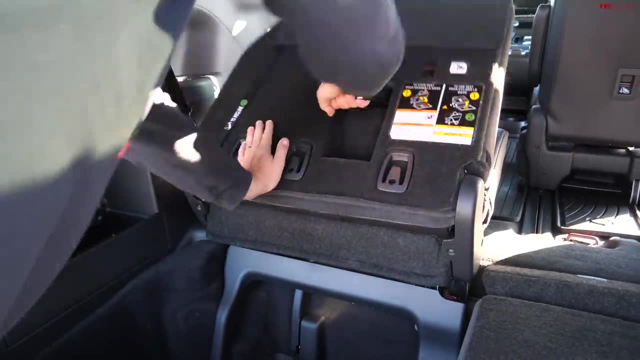 Okay, Yeah, So go ahead and open it. The opening thing is easy. Just follow the instructions right there. So go one. Sorry, I'm not good at following. It's terrible at following the instructions. There you go. Yeah, it's pretty easy. 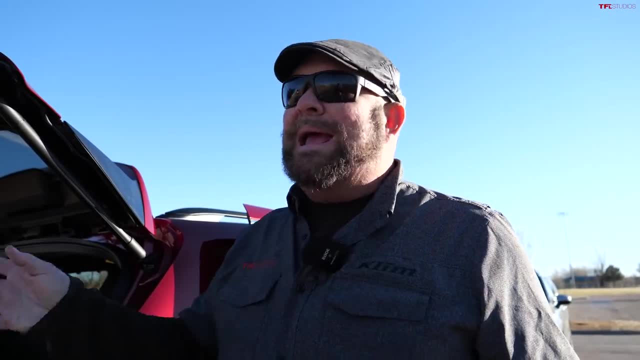 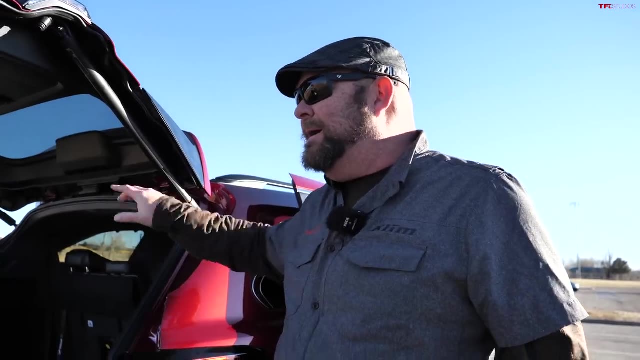 All right. Now a big question about, first of all, cargo room and the ability to pull A four by eight piece of plywood, or something like that, from inside of here. Okay, There's a problem. What? In order to do that, you have to have the seats folded as much as possible. 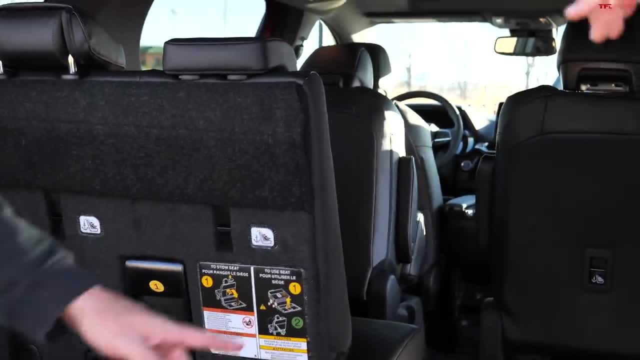 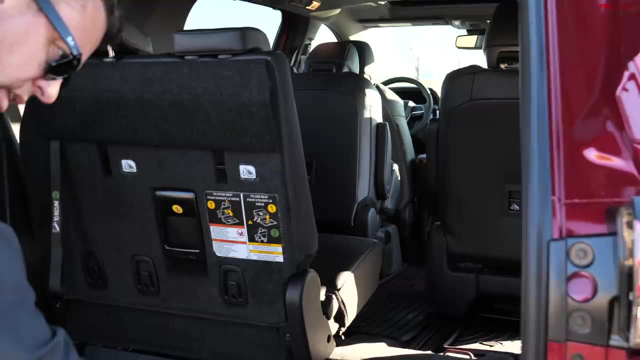 And most likely, the plywood is going to have to go in at a bizarre angle near the roof, And it probably Is that because of the captain chairs- Exactly Those captains chairs are not supposed to be removed. Okay, If you look, what's the width of the opening there. 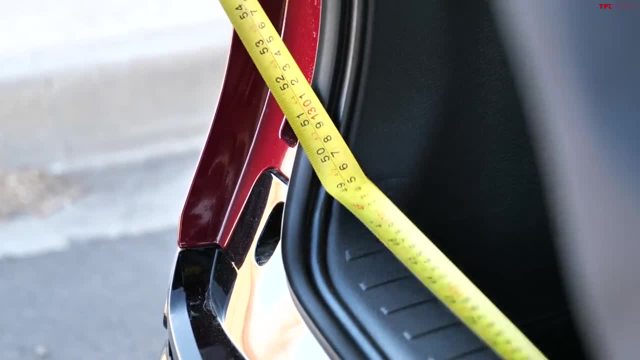 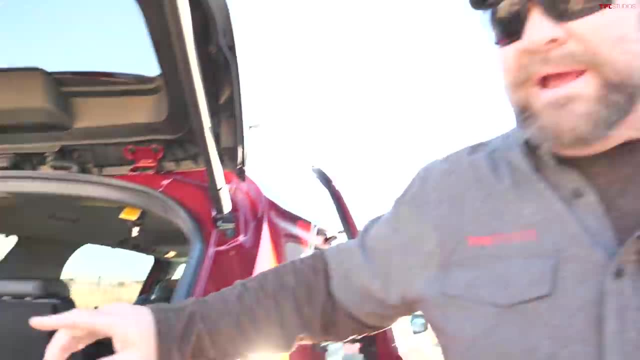 It's like 49 inches, because so that's so a four by eight would fit. Yeah, That way. Width wise, Yes, But not length wise. Okay, At a really weird angle to work, Tell me about the cubic footage here. 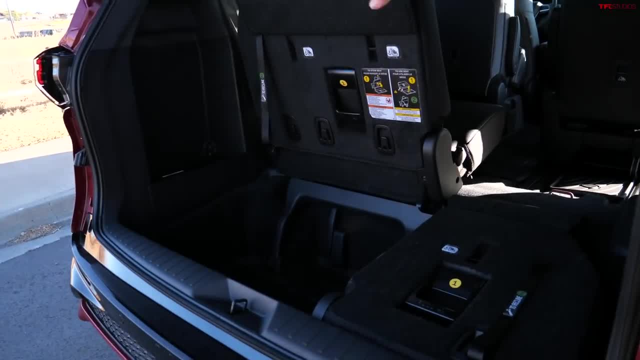 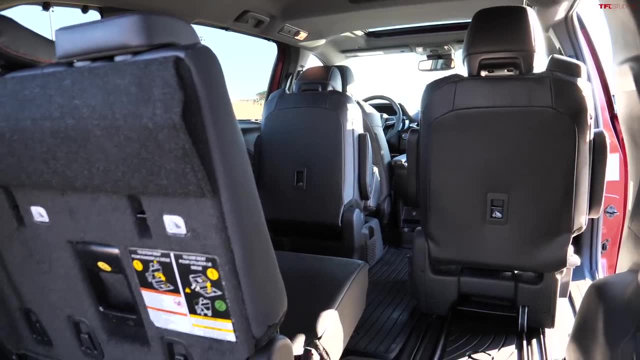 33 cubic feet back here behind these seats. Okay, Fold these seats down and you move the center row all the way up. 101 cubic feet of cargo space. Okay, What about the Kia? Ah, let's have a look. Actually, this opening is a smidge smaller than the Toyota's. 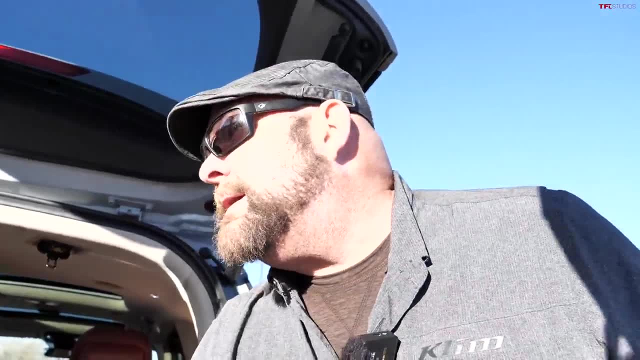 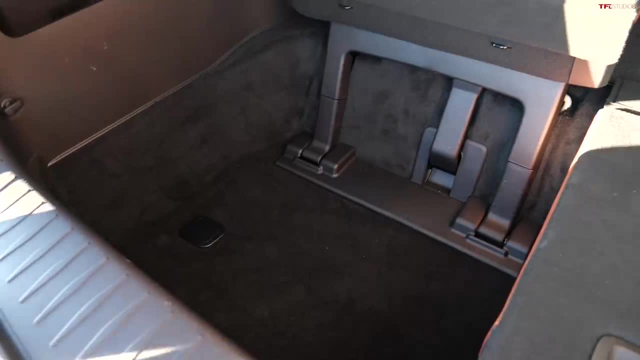 Yes, That's interesting. And on top of that, this opening down here is bigger because this is 40.23 cubic feet of space, So it is Behind the third row. Yes, Okay, What happens if I can do this? 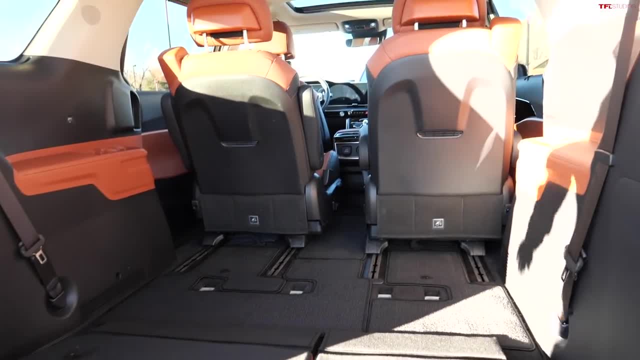 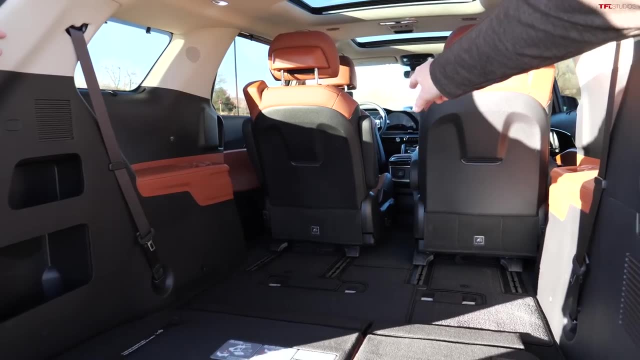 What happens if I do this? Ah, then it moves up to 145.1 cubic feet of space, Once again, more than the Toyota. But once again, these seats are not supposed to be moved out of there. There's airbag issues and safety issues should not be moving these out of here. 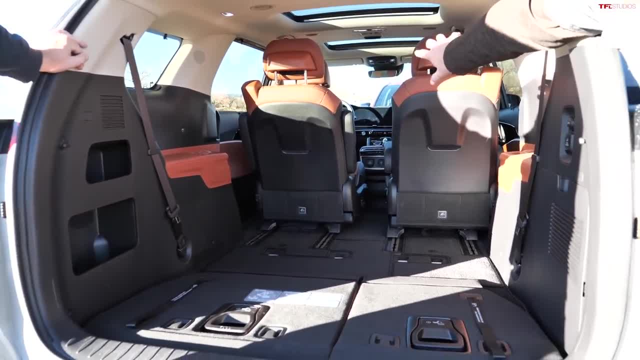 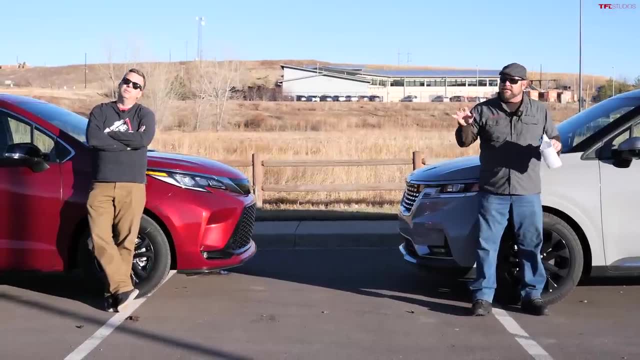 So you can fold them forward as far as they'll go. You can fold them slightly down. So if you're putting a four by eight sheet in here, it's going to have to sit at a weird angle. Just so you guys know, there are various trims for both of these vehicles. 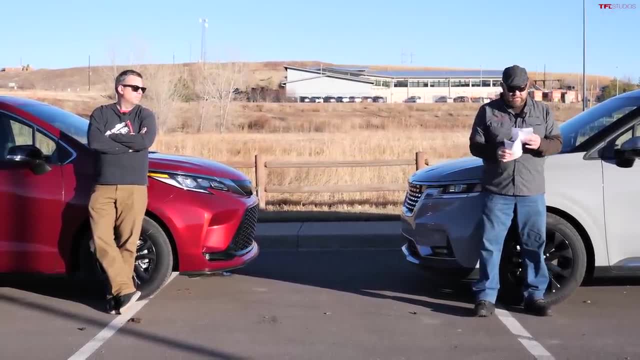 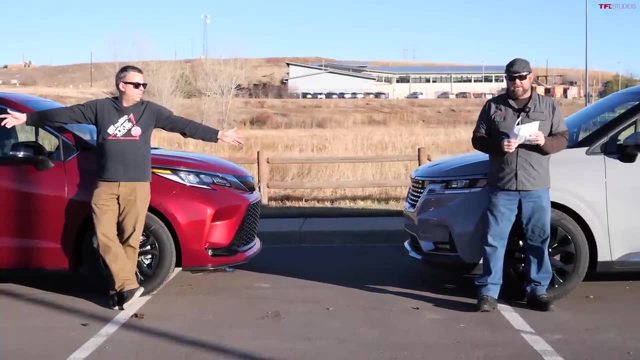 And the starting prices are lower than what we have here on the stickers. So for this, Sienna base price, front wheel drive: $37,185.. Good luck finding one of those. What's the base price on the Kia? That's an excellent question. So the Kia comes in at $33,200 for a base price. So that's almost like $3,000 to $4,000 difference. Yeah, And that continues. So there are a bunch of differences, So there are a bunch of differences. 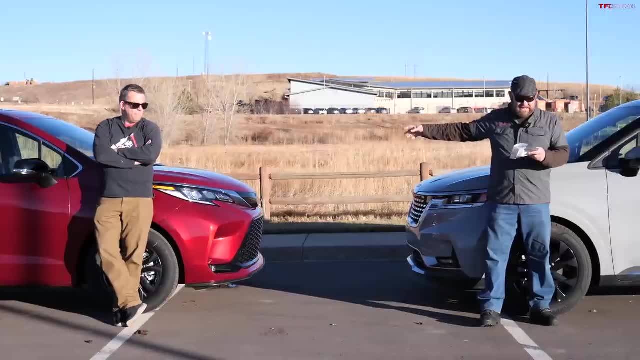 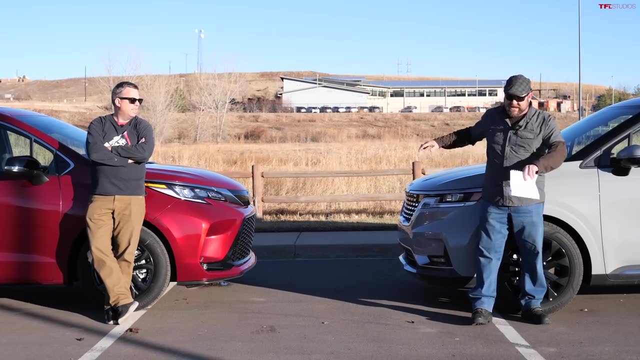 So there are a bunch of differences, There are different trim levels, obviously, So that one, for instance, the LE, the XLE, the XSE, the woodland edition, It goes all the way up. This one, the LE, the EX, the SX, the SX Prestige. 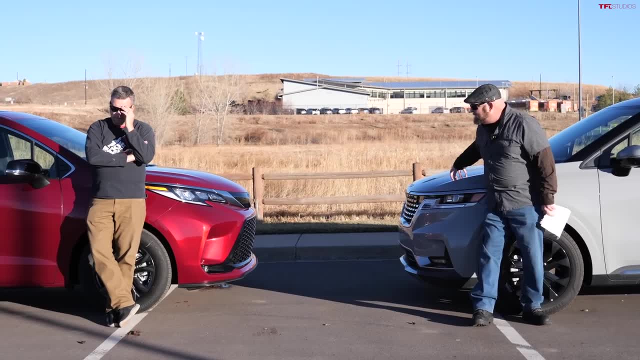 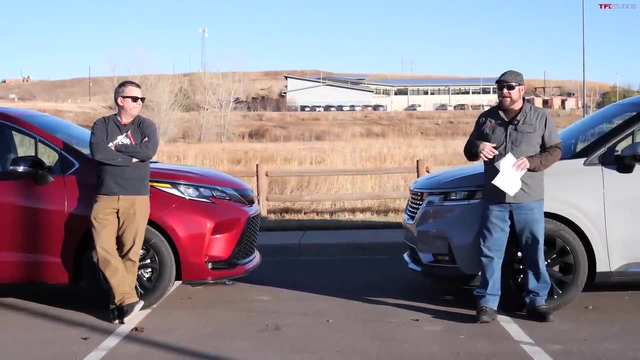 That's what you're looking at here is the Prestige. So this is very top of the line And that one is sort of a mid-level right. That's where the big pricing difference comes in, And I think part of that is the powertrain, because that's super advanced. 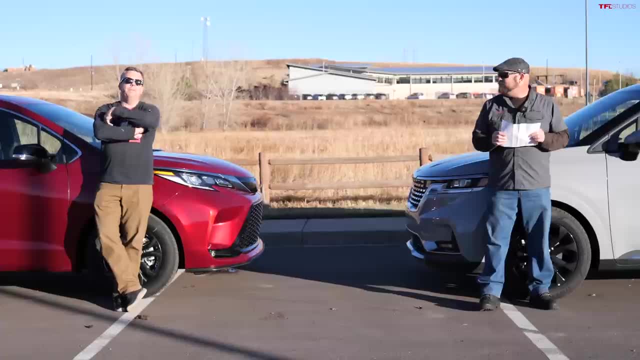 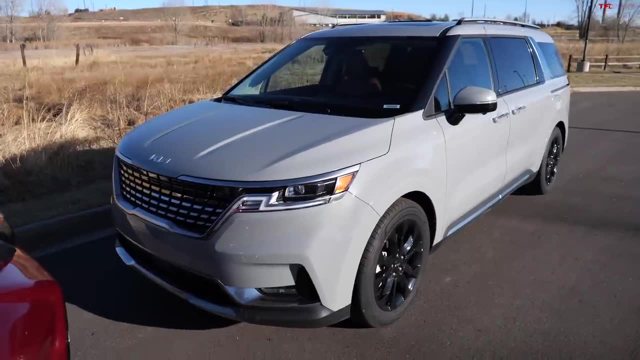 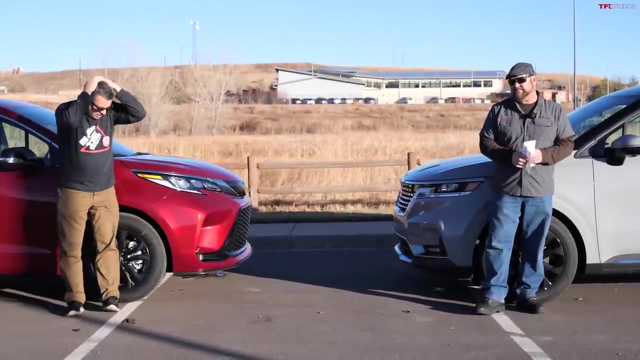 So, as tested, this Sienna Overdrive XSE is $52,374.. All right, As tested, this 2024 Kia Carnival SX Prestige comes in at $49,480, the MSRP. So I have a problem, Yeah. 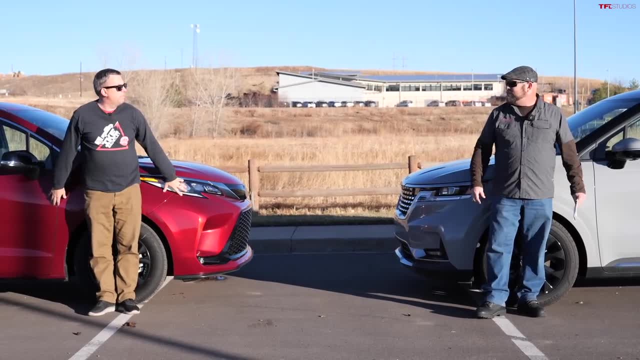 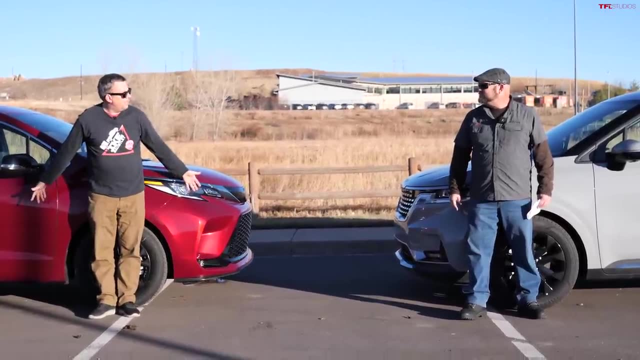 Because all this video? I really love the efficiency of this van- Yeah, I would agree. And also the usability is not bad. No, not bad at all. But you're telling me this is like three grand more, It is more expensive.